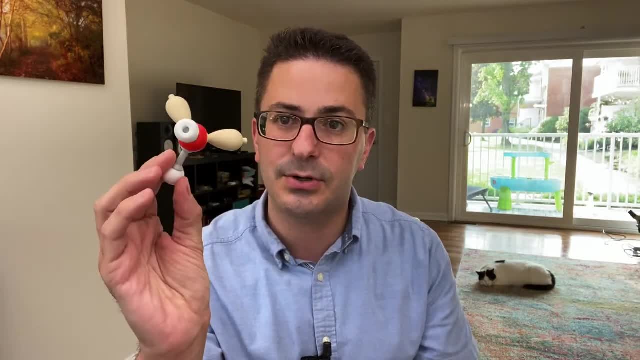 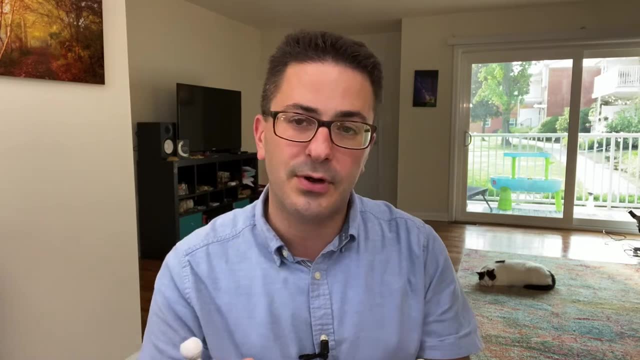 Here are the four-holed oxygens, the lone-pair electrons and the two-holed hydrogens. What this allows us to do is it allows us to model hydrogen bonding, which is very important for organic chemistry and biochemistry. Here's another molecule. This is called isopropanol. This is what 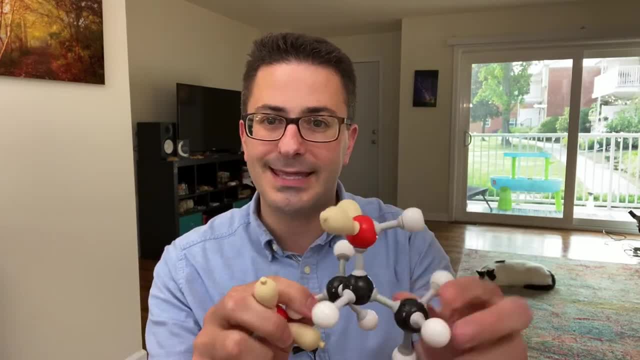 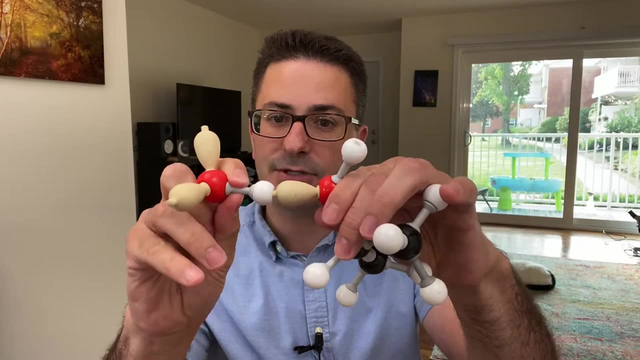 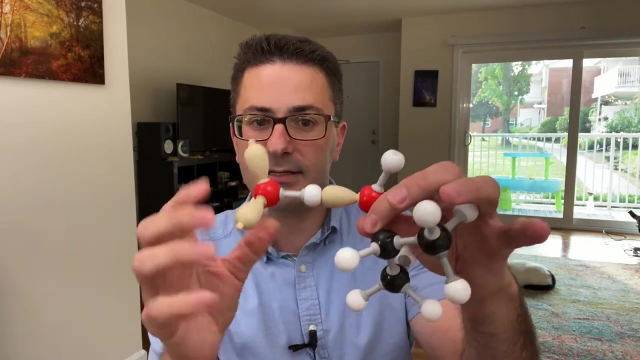 we use in our hand sanitizers. now, Isopropanol is miscible or it can dissolve in water. The reason that is is because both molecules can hydrogen bond with each other. Because water and the alcohol are similar structures, we get this kind of interaction. The reason it exists is because the 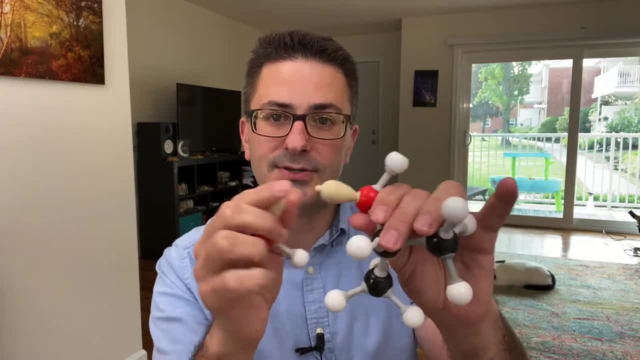 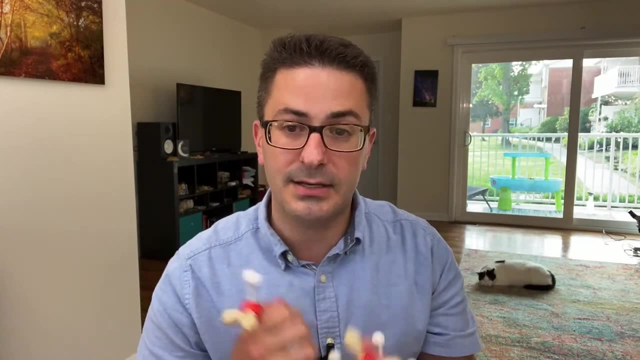 proton is a little bit positive charge because it's polarized, and the electrons are a little bit negative. So positives and negatives attract and you get this hydrogen bond. We don't really have the ability to do that in any other way other than through this special kit and many of the lessons. 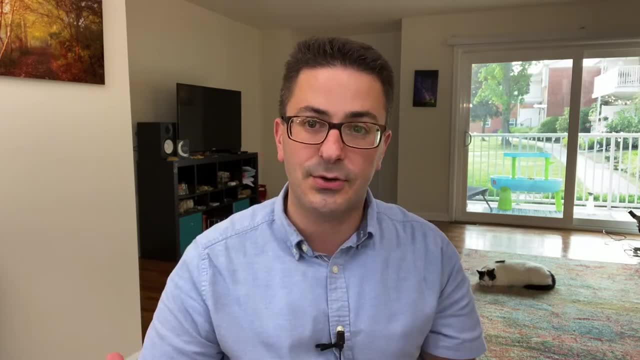 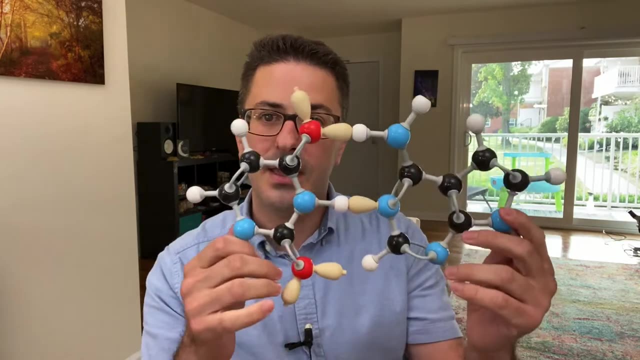 use this. We have special lessons on hydrogen bonding. It kind of permeates all of biochemistry. Let me show you one other really cool application of hydrogen bonding which a lot of people even know about. They don't realize they know about it, but this is a DNA. 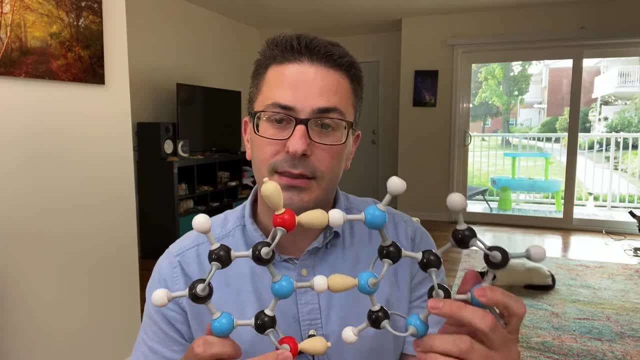 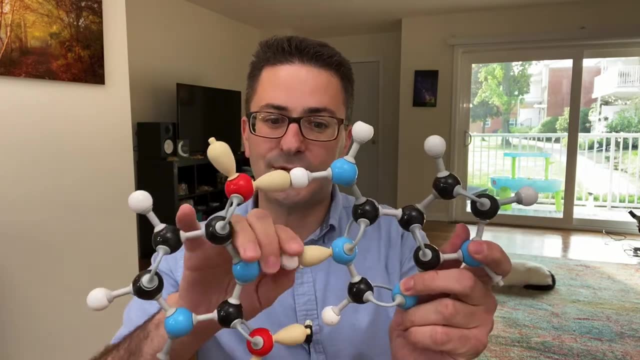 base pair. Everyone's heard of DNA base pairing. What's causing the base pairing? Why do the A's and T's and the G's and C's, why do they base pair with each other? It has to do with hydrogen bonding. So here I have these hydrogen bonds formed already. I'm going to unform them. I'm 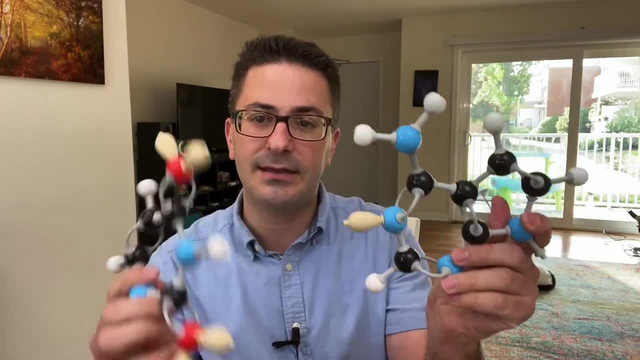 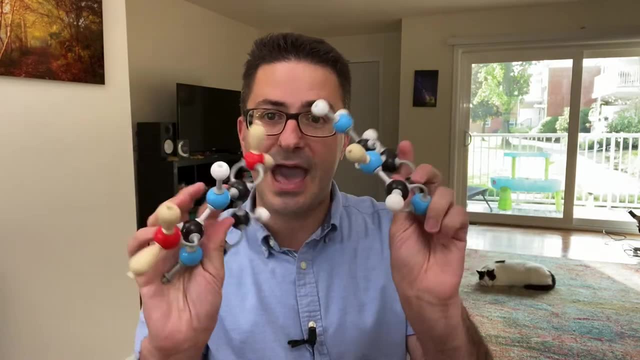 going to melt them. actually, Now we have two. Now we have the adenine, and this is actually a uracil, which is the base we get in RNA. So the students have, by the way, they have, enough pieces to build this model. That's. the other thing with the kit is that they have enough pieces to build. 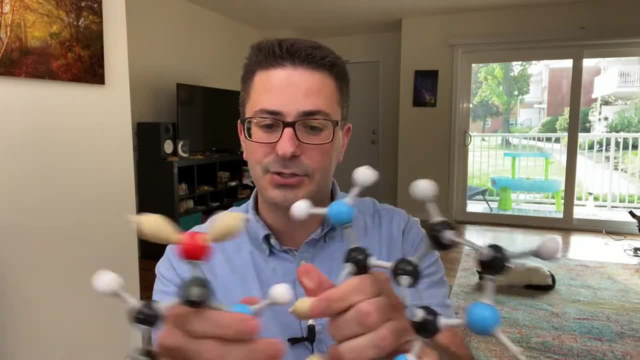 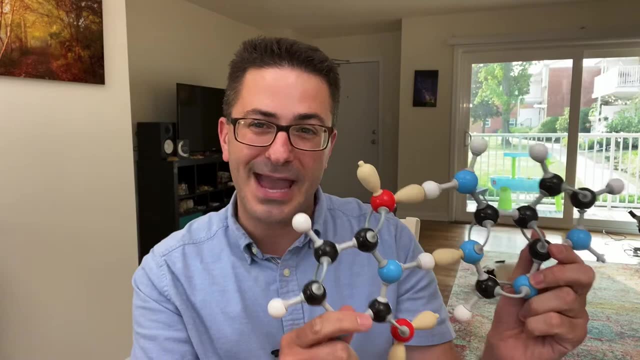 this model. We don't know how many of the molecules that are in the curriculum, but we can model hydrogen bonding, We can model base pairing through this sort of interaction right here, And by the time the students get to this exercise they completely understand what's going on. So 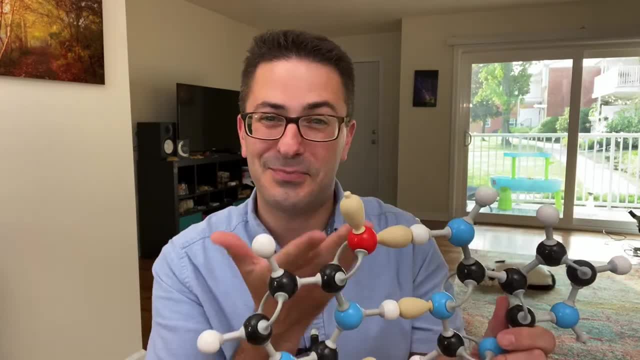 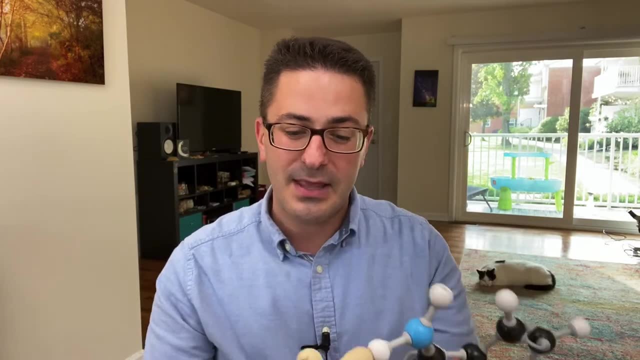 I don't expect most people watching this to get everything other than the fact that we're seeing hydrogen bonding, but they really do understand what's going on and add so much to the curriculum to have that ability to do that. The other important piece that's in the model kit are these: 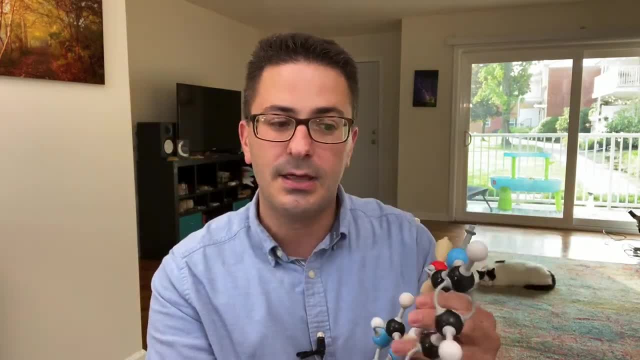 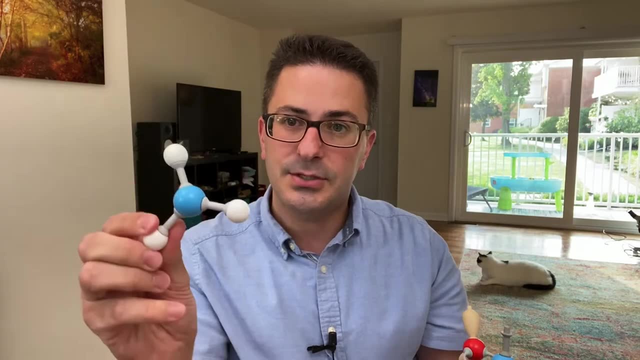 special nitrogens that have only three holes. Most of the kits from Mollymod are for organic chemistry and they'll have four holes, so they'll look kind of like this. We need the three-holed nitrogen to model a concept called aromaticity. 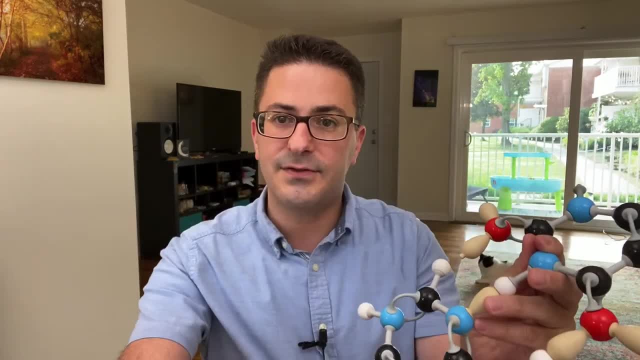 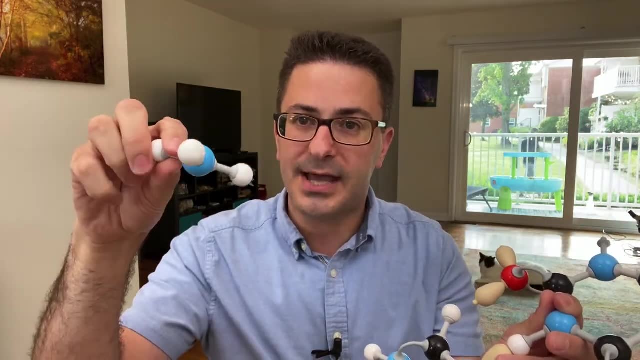 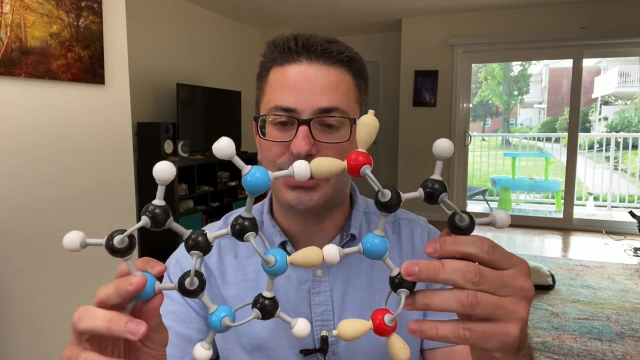 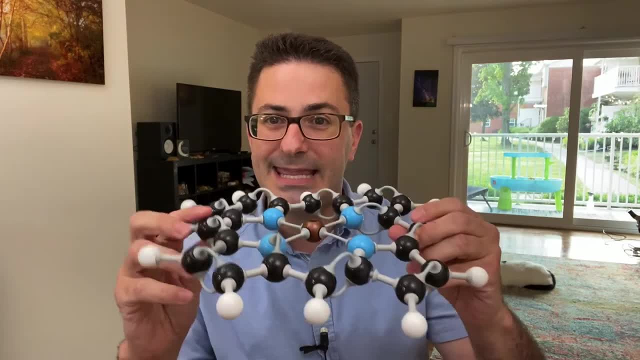 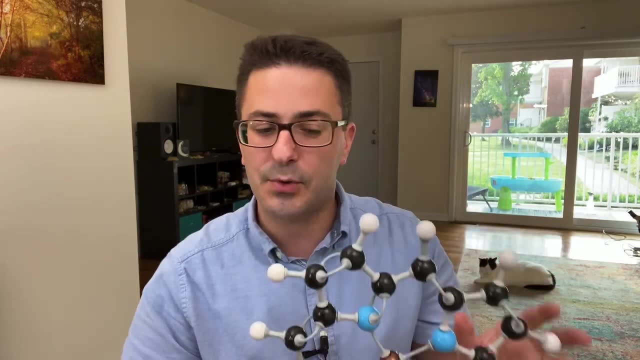 We're going to use a molecule that's very flat. We're going to use a molecule that's very flat That is also found in many other molecules, for example, the heme of hemoglobin. The kit doesn't have enough pieces to build this, but if you have a school subscription, you would have more kits. 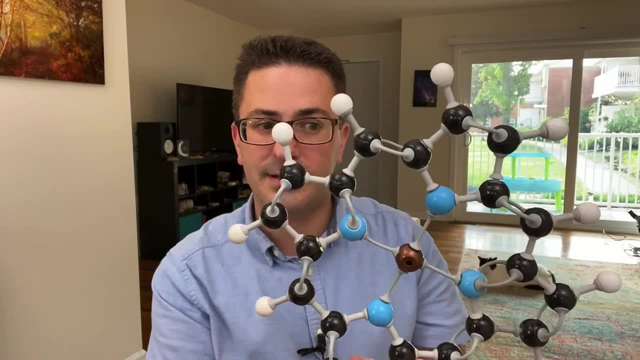 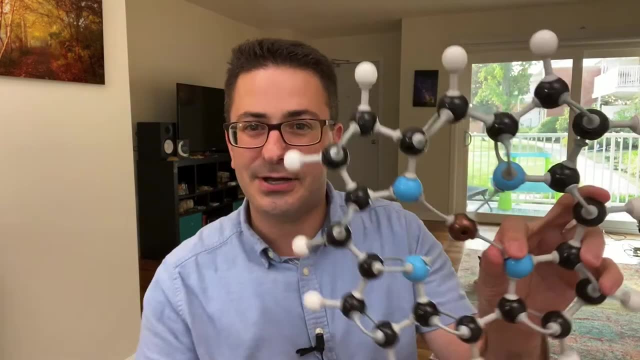 around and the teachers could build something larger like this porphyrin molecule, which is from the heme of hemoglobin. Let me just show you one other cool application of hydrogen bonding. In the center of this heme we have this very important iron. That's the iron in our blood, The students. 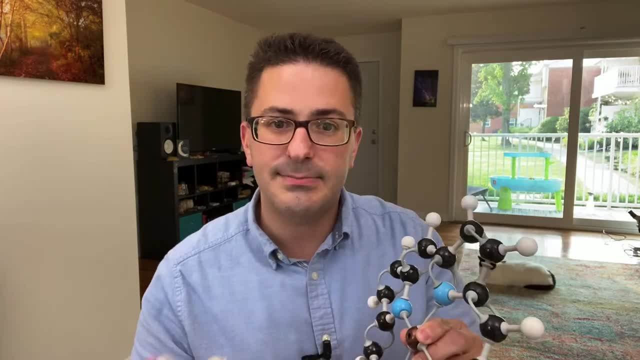 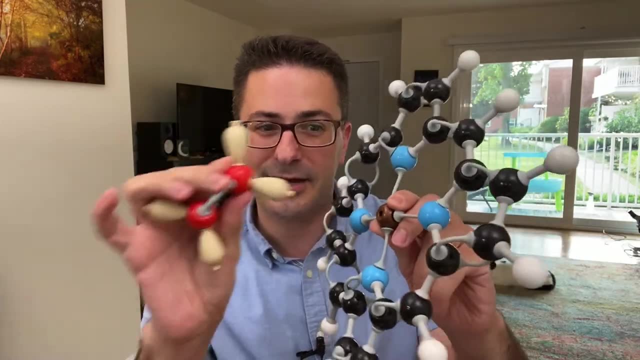 learn in the ionic chapters that iron tends to be a little bit positive charged. Those lone pair electrons are negative charged. So when we breathe in oxygen, what do you think happens with the oxygen and the iron Sticks together, We're actually seeing the biochemical basis for 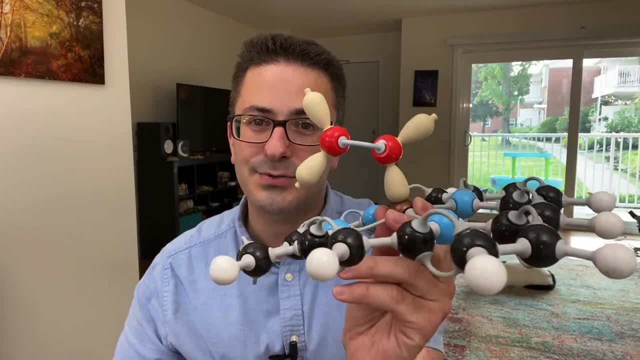 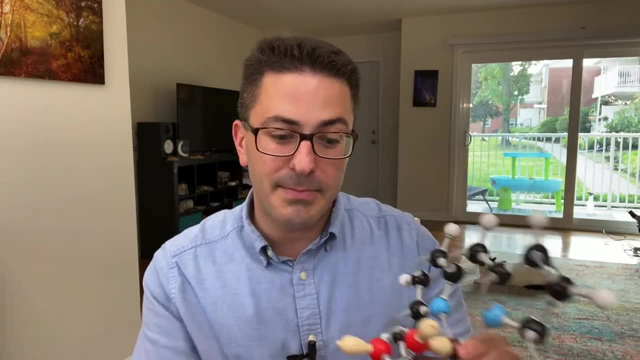 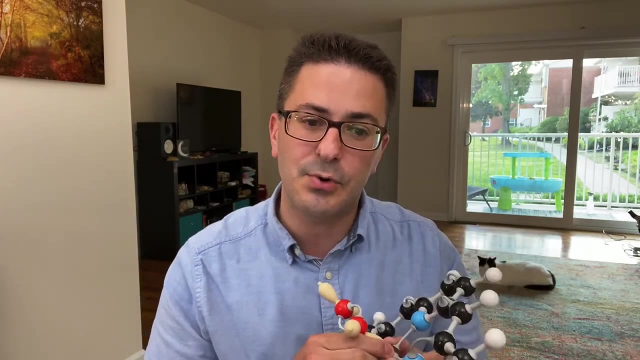 breathing. Where does the oxygen go when we breathe it in? It goes right onto that iron in our hemoglobin. So it's really cool to see these applications in the model kit. We can kind of have the students easily model them, and the way that it kind of sinks in is just so much more beautiful when we have the ability to look at. 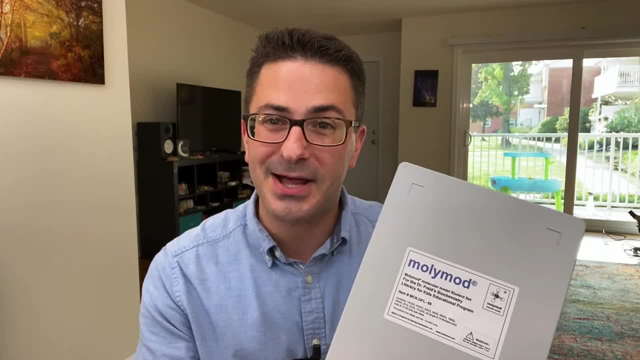 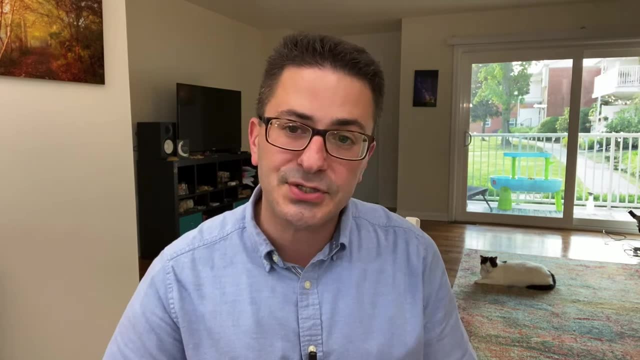 hydrogen bonding. So, anyway, that is the custom Mollymod kit that is produced in collaboration with Mollymod. You can't get it anywhere else. You have to get it through the website. There are other options for you If you are outside of the United States or maybe too far. 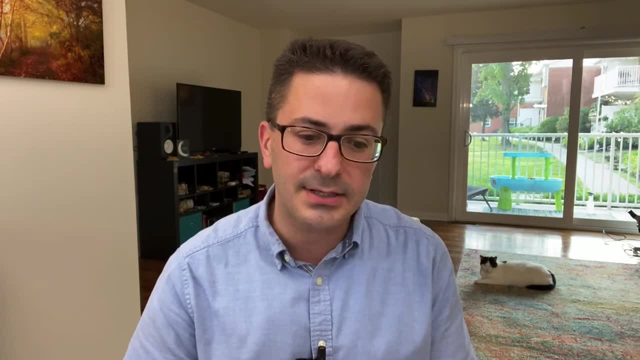 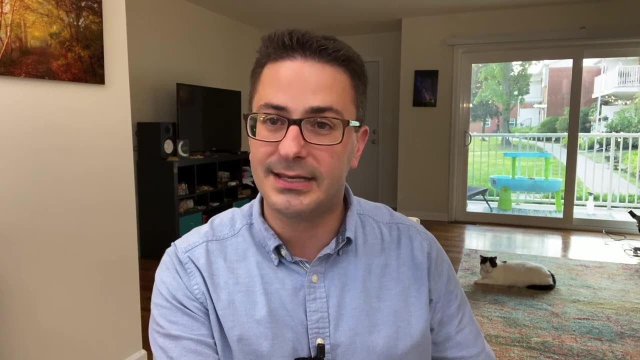 from England, which is where these are produced. you can order other model kits and you'll do just fine, But if you can get your hands on this kit, I recommend it. The program is designed for this kit, so it's really just worth it to have it. Thanks,